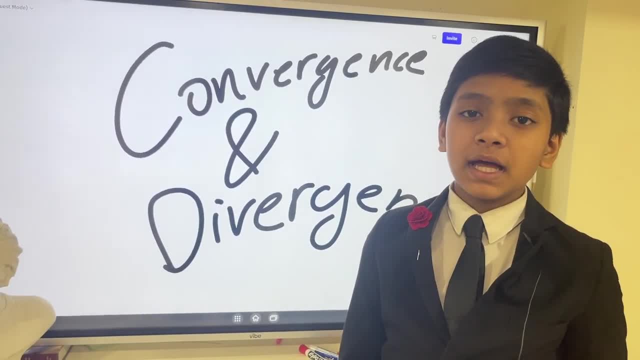 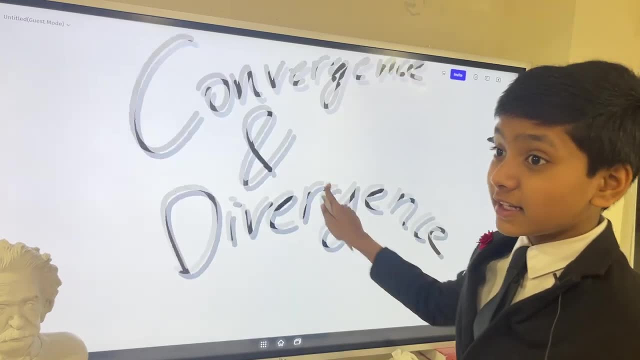 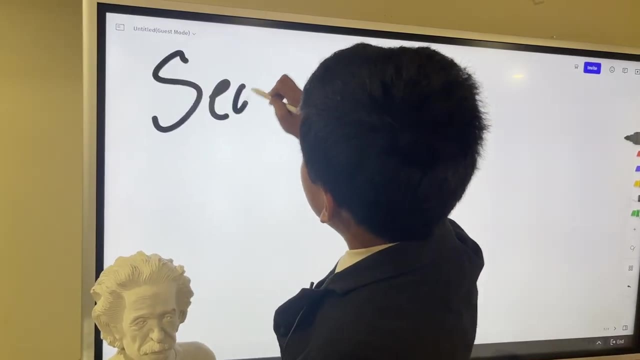 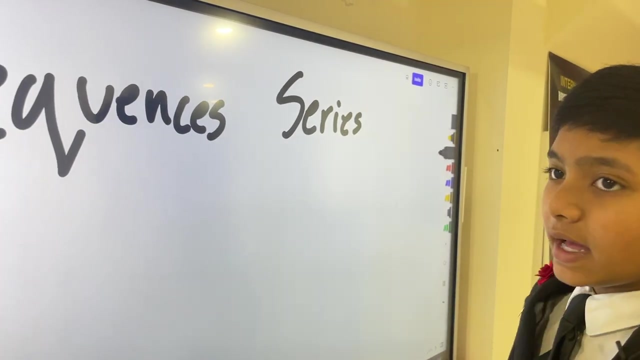 Hello everybody, My name is Ibono Logicberry from Mary's Science Lab, and today I will be talking about convergent and divergent functions. No, not functions, but technically functions. So today we're going to be talking about sequences, series and how that all relates to functions being convergent and divergent and all that. 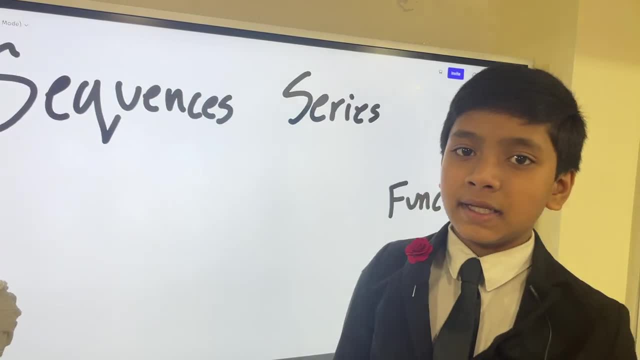 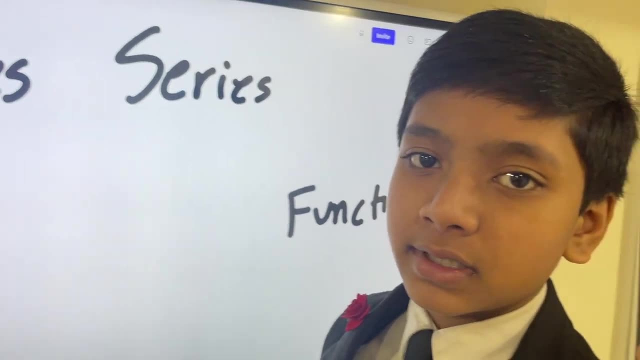 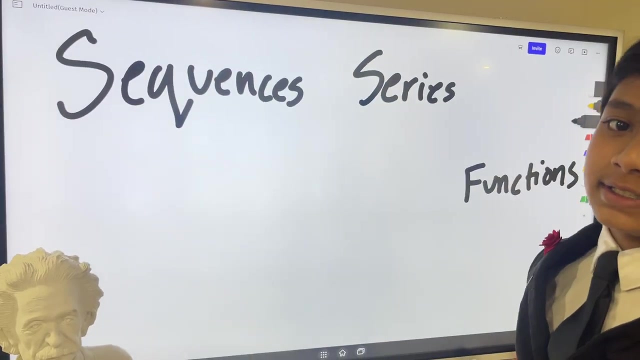 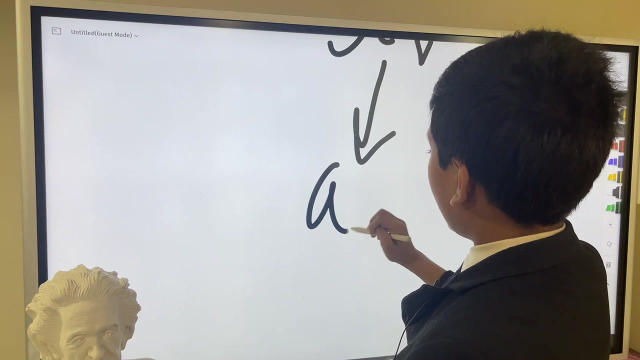 And a prerequisite for this is basically, I guess, derivatives. So basically, you've got to know how to take derivatives and limits if you want to understand this, But that's not too bad of a requirement. So what are sequences in series? Well, they're pretty simple. Let's take a sequence like I don't know, an equals. I'm going to pick something like 5n. 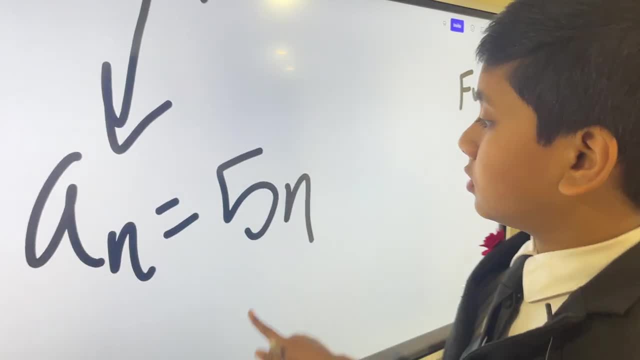 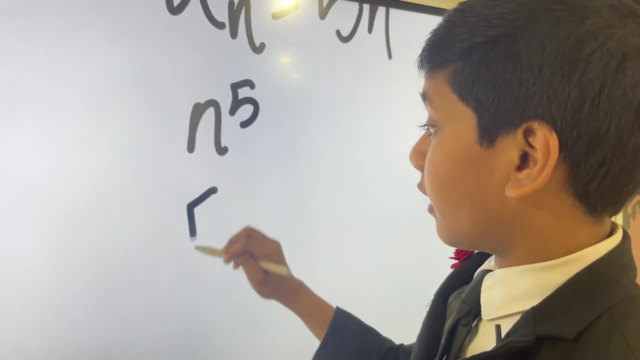 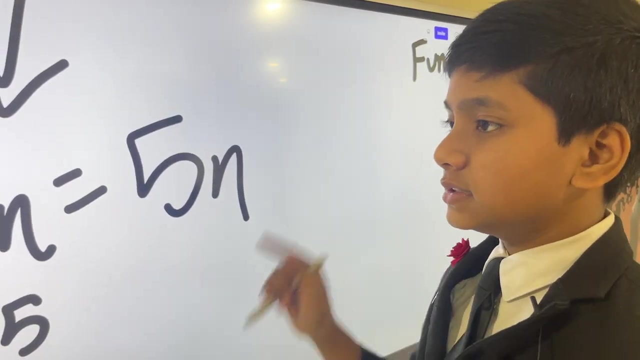 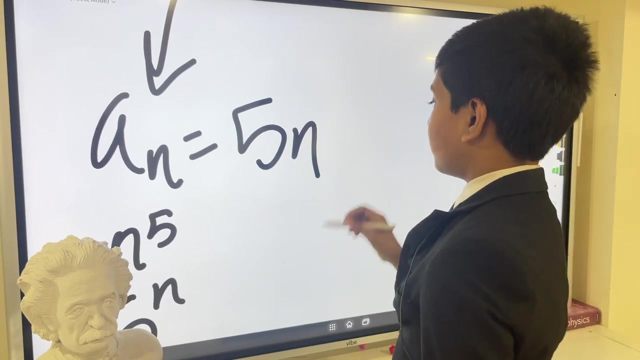 Or it can just be anything relating to n, So like 5n, or you could have n to the 5,, which would grow very rapidly, Or you could have 5 to the n, which would also grow very rapidly. So just so I can stick with something I know and I don't fry my brain trying to calculate values, I'm going to start with 5n, So let's list the values. 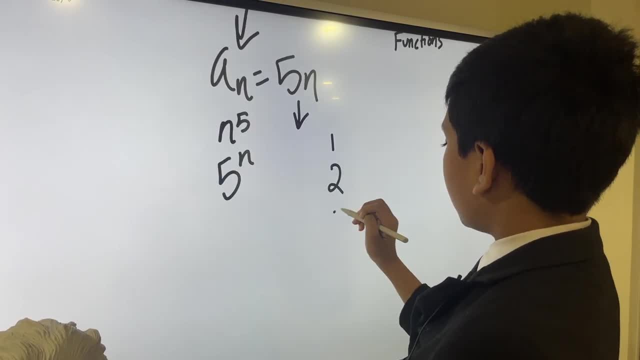 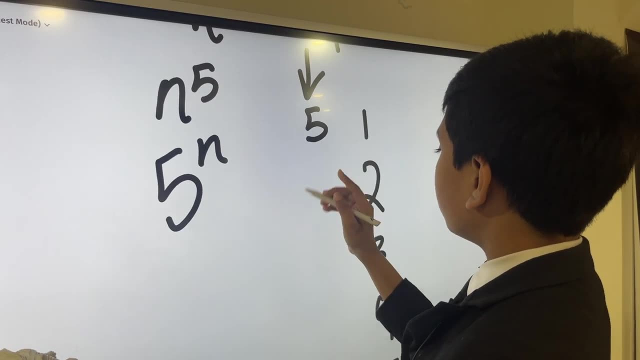 Term 1, term 2.. Term 3, term 4, term 5, so on: Term 1, 5 times 1, 5. Term 2, 5 times 2, 10.. Term 3, term 4,. you probably get the deal. 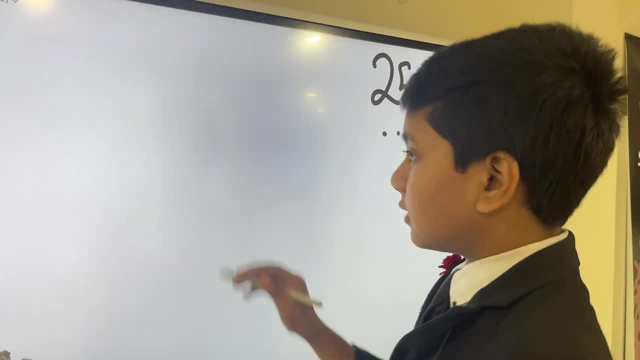 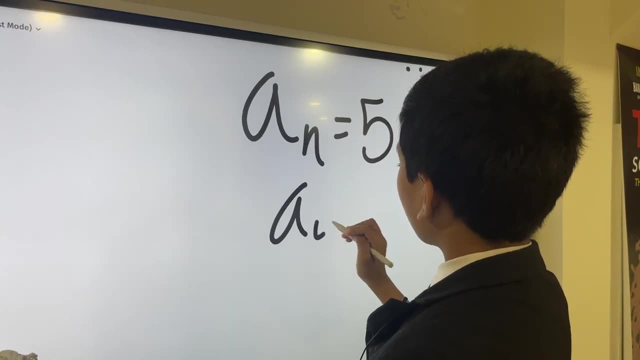 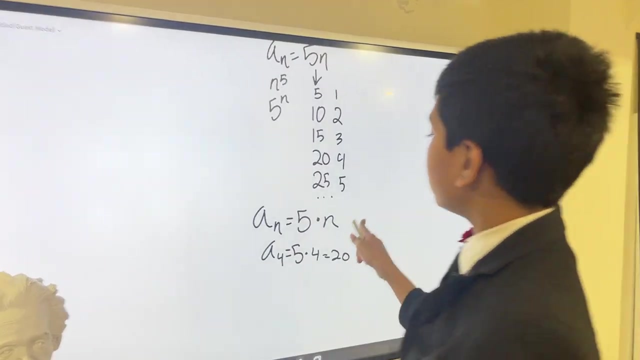 This is going to continue on and on. So something like an is just going to be 5 times that number, n a4 is going to be 5 times 4, or, in this case, 20.. So now, what is a series? 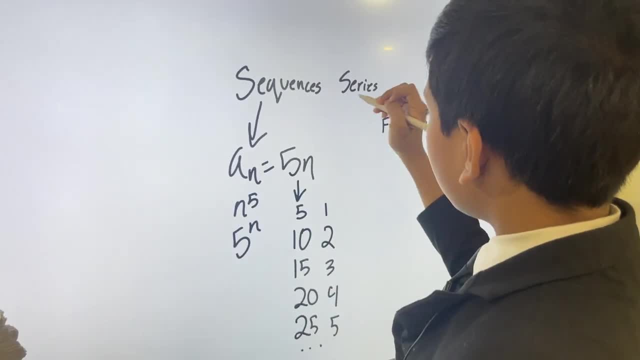 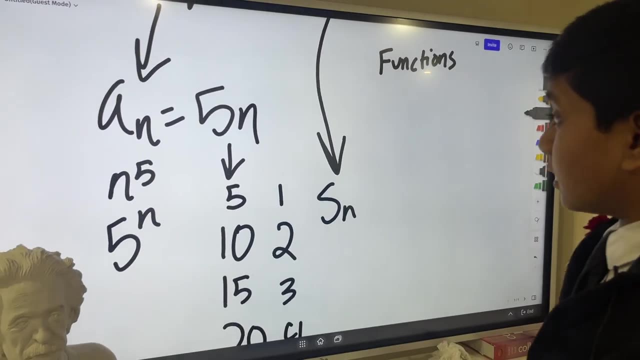 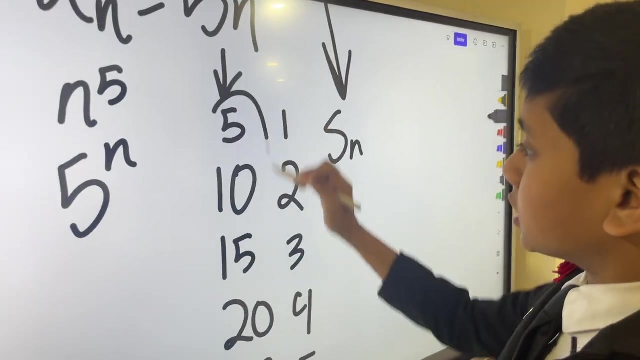 How is it different from a sequence? Well, series is represented by s of n and it's not like a series and it's not like a sequence that, instead of having all these terms, it adds up a certain amount of them. 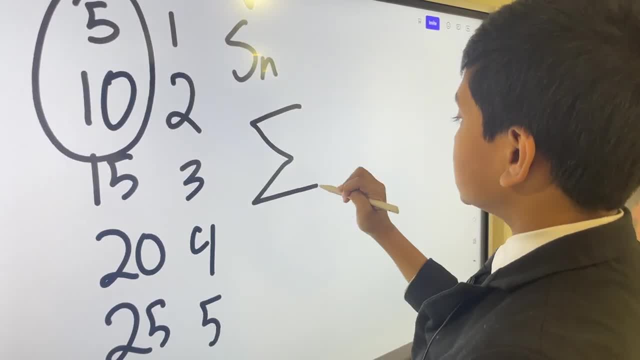 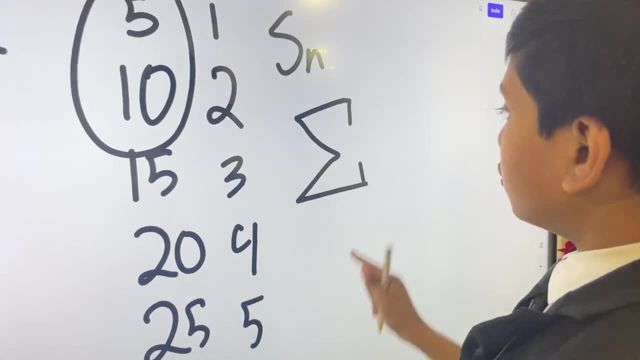 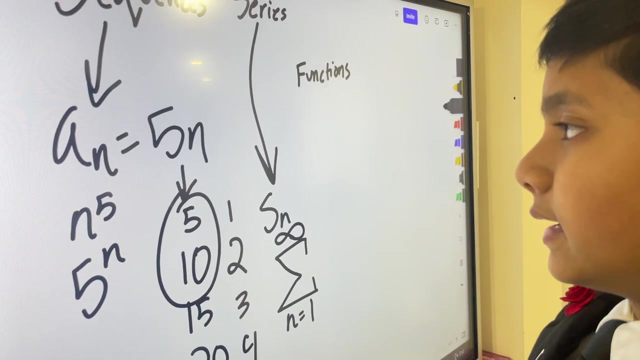 With this notation that we call sigma. I'm lazy, but most people. I'll add these little two lines on the end of the sigma So you can basically put this: from n equals 1 to infinity and then express it for your sequence like 5n from before. 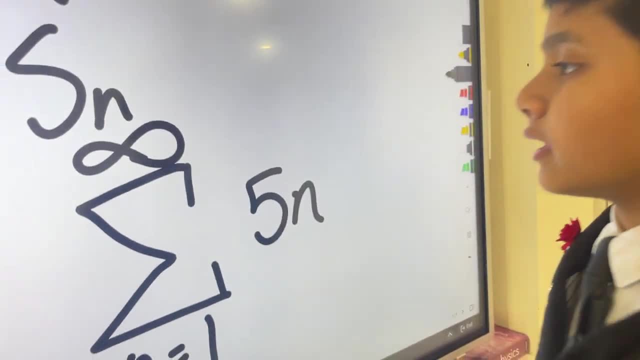 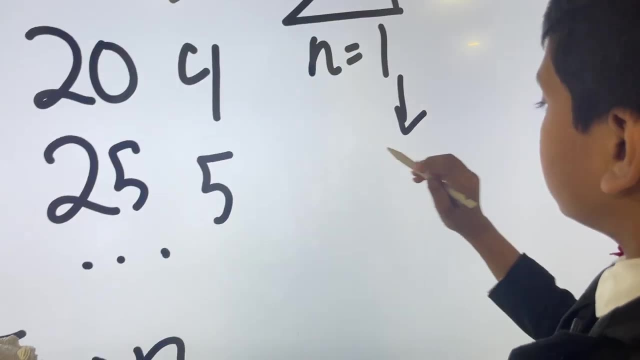 This is basically saying it's summing up all the values, from n equals 1 to infinity, or in other words, it's summing up all the terms, So it's doing 5 times 1 plus 5 times 2 plus. 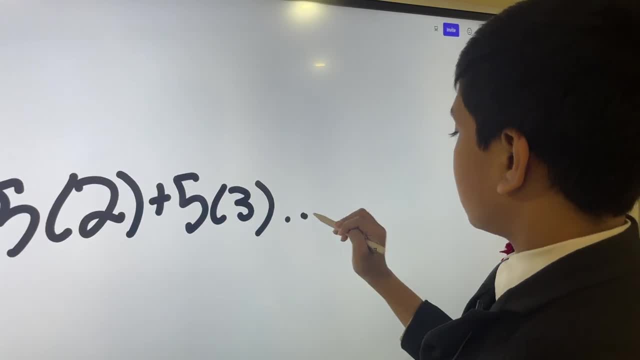 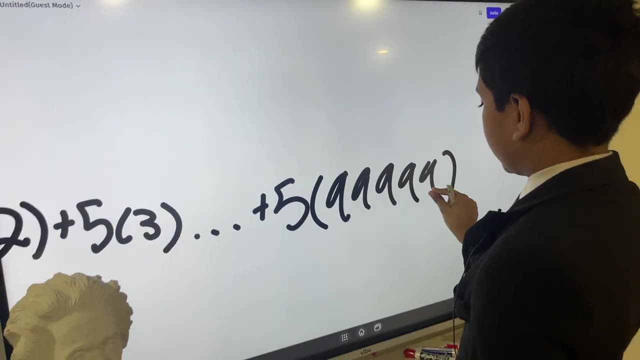 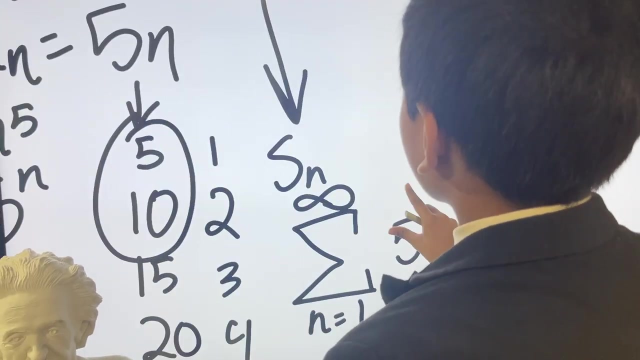 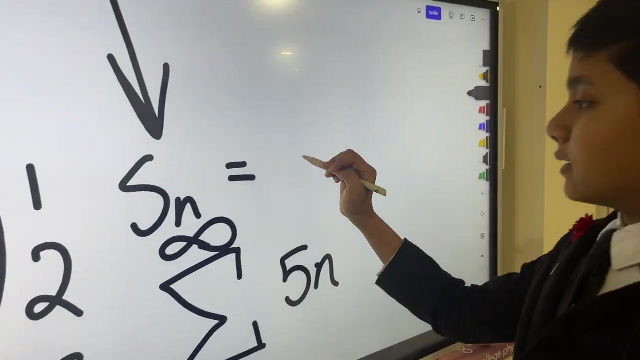 5 times 3. All the way to infinity. So you could put like some very large number on the end. I don't really care. So this is a sequence. It's adding up this number of terms. Or another way to describe it would be saying: sn would basically be equal to an plus, an minus 1, an minus 2.. 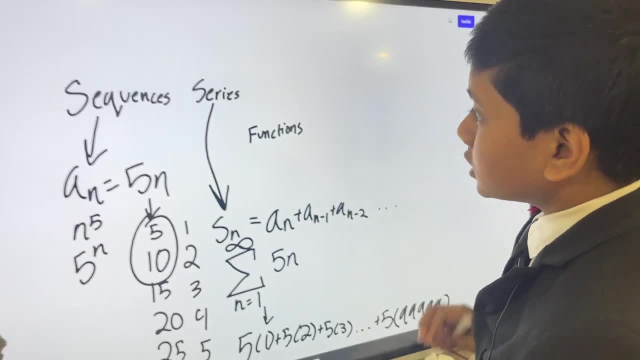 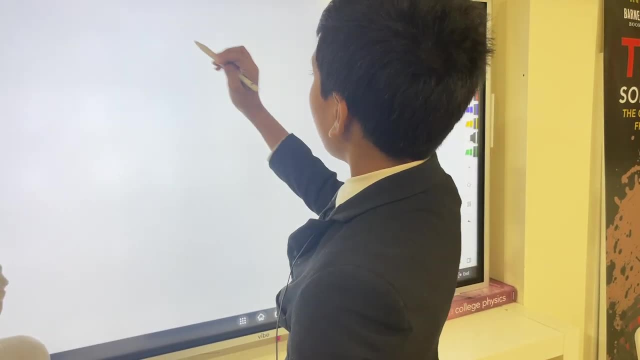 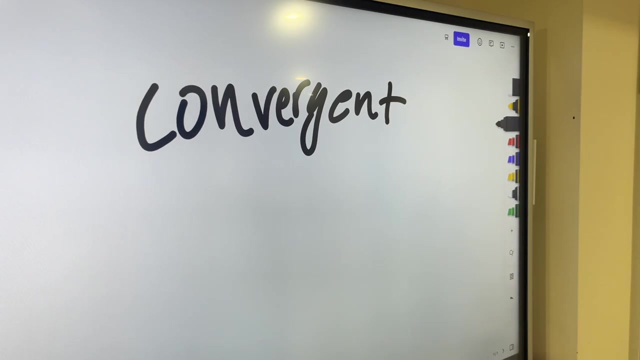 etc, etc, etc. Alright, So what does convergent and divergent mean? Well, you probably already know what convergent means. Name is self-explanatory. It basically means that the sequence s of n as n approaches infinity. 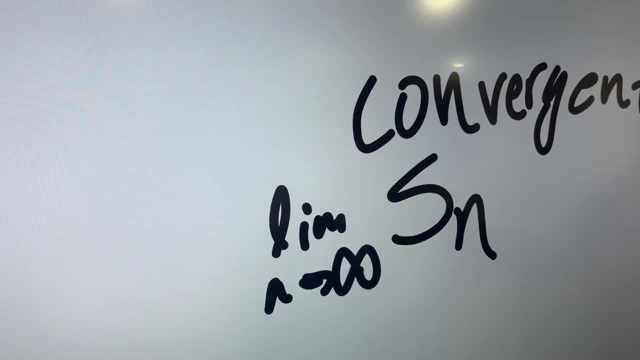 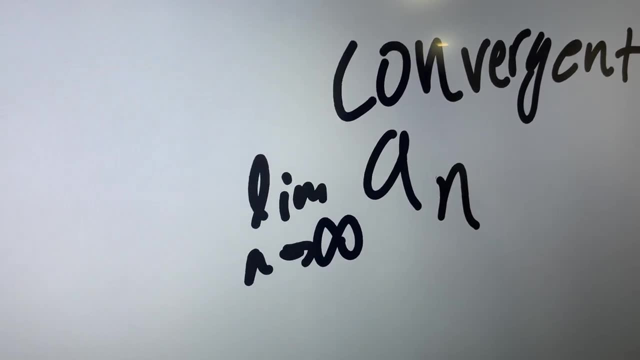 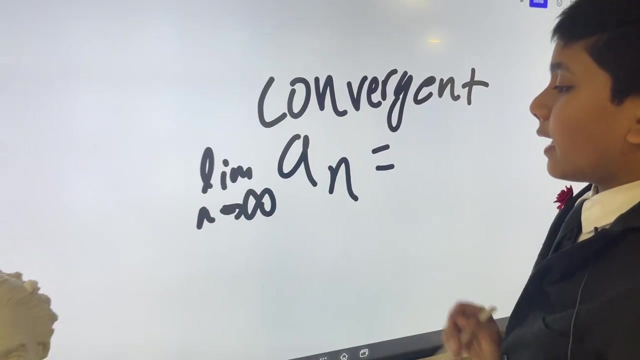 Well, you can't really take the limit of the sequence. So, more than that, it's a sequence. So more than that, it's a sequence. Or like, as n approaches infinity for a sequence. I keep getting the name of sequence and series mixed up. 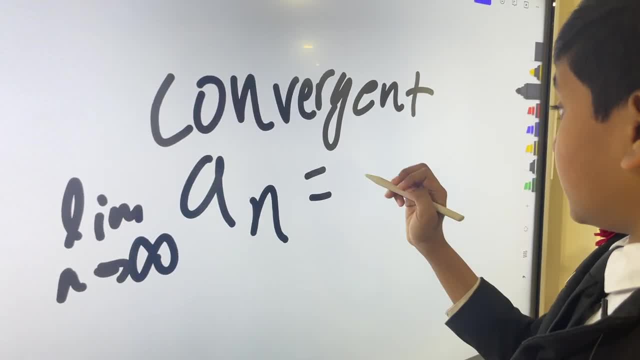 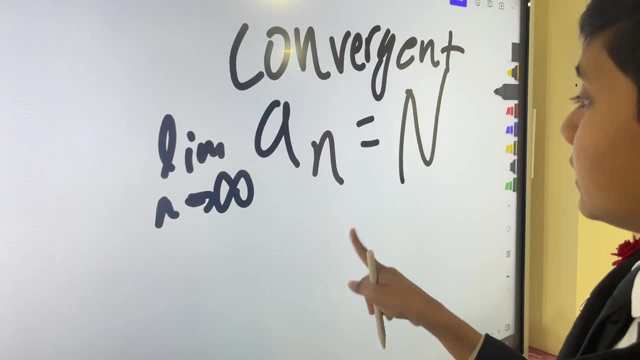 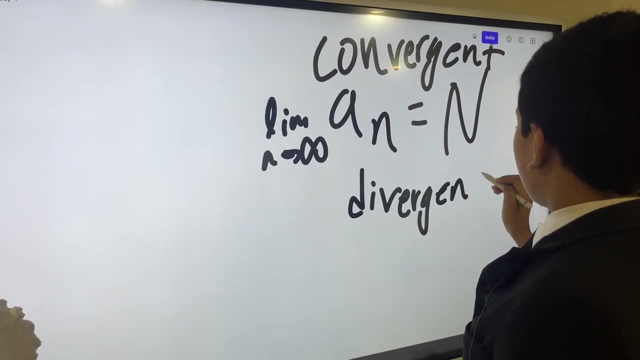 If it's equal to some constant, we can call it- I guess, I don't know, n. If it converges it's some constant, then that's what we call convergent Divergent than be any one of three results. 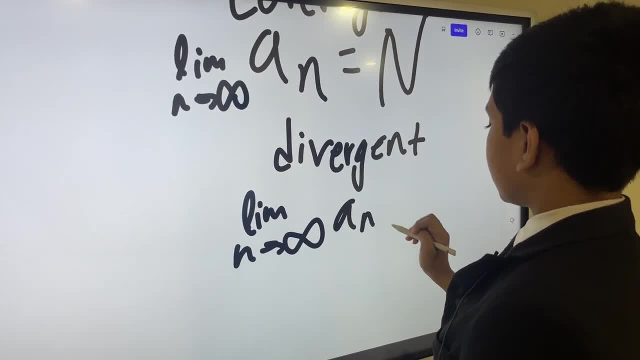 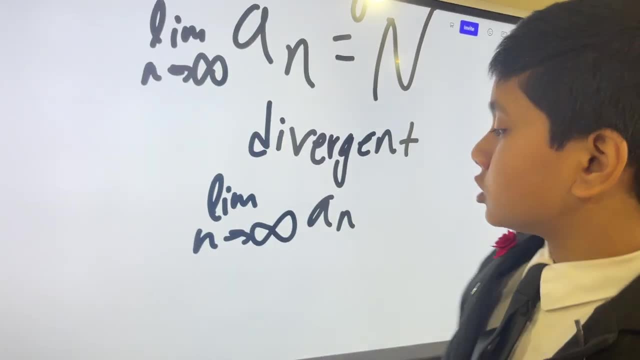 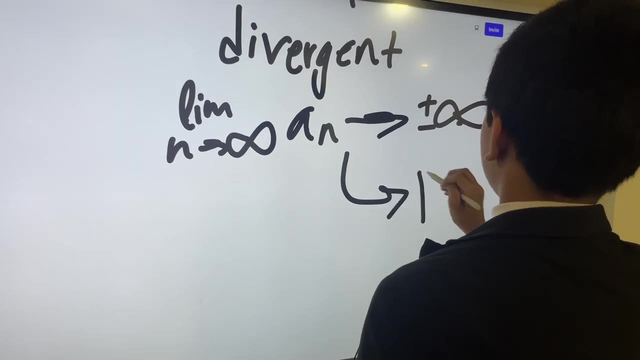 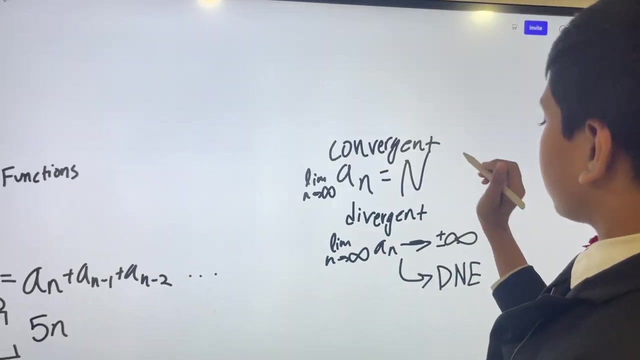 Or two results. I guess It basically means when you take a limit and it approaches infinity. so basically, when your n gets very, very large, a of n gets either one of the infinities or just simply does not exist. Okay, so those are how we do convergent and divergent. 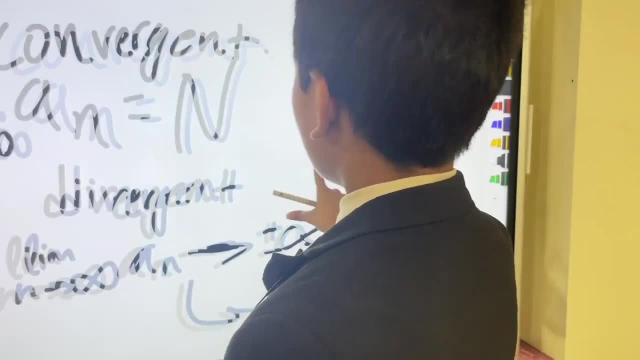 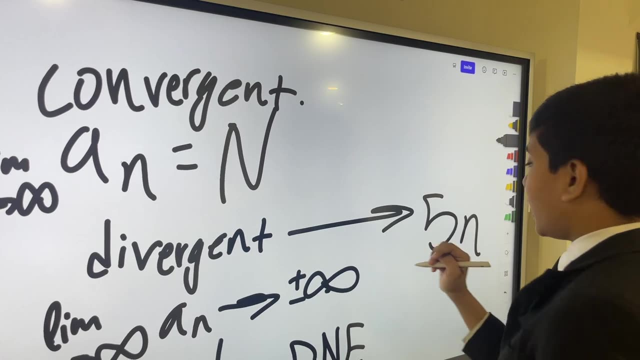 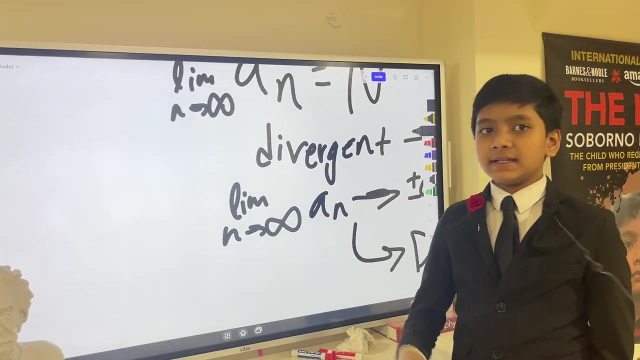 In fact, let me show you two examples. A divergent one would be something like: oh no, the example that I just showed you, 5n. Why? Because think about it. This is basically talking about when the terms get bigger and bigger and bigger. 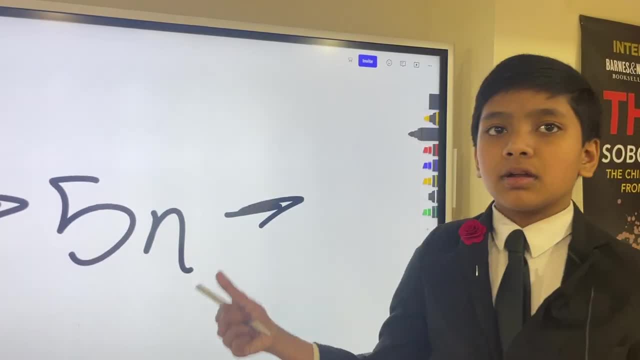 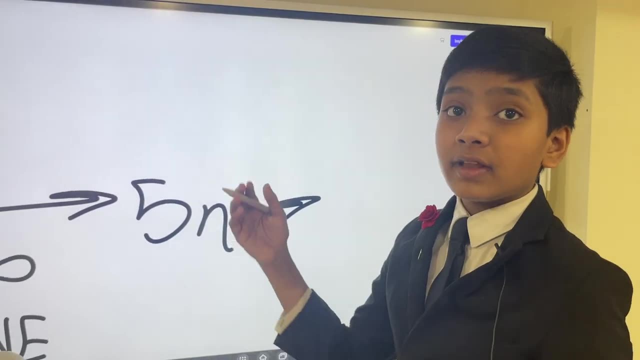 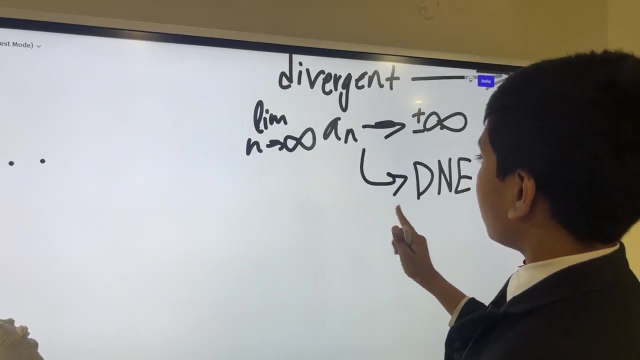 I mean there is no place where the answer to this stops growing, right? I mean, it keeps growing. it keeps growing because you add 5 to every term. The amount you add never decreases. So in other words, you could also say that: 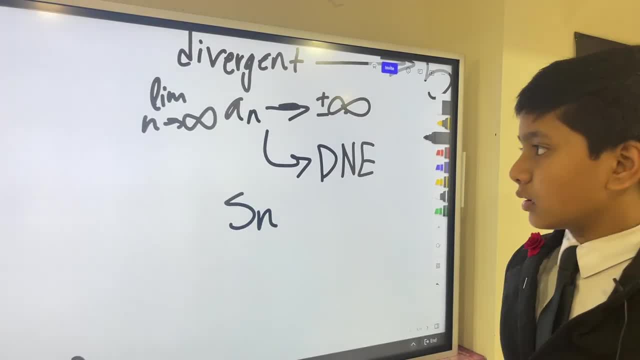 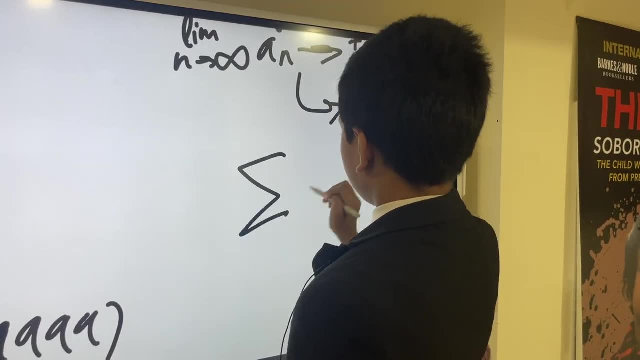 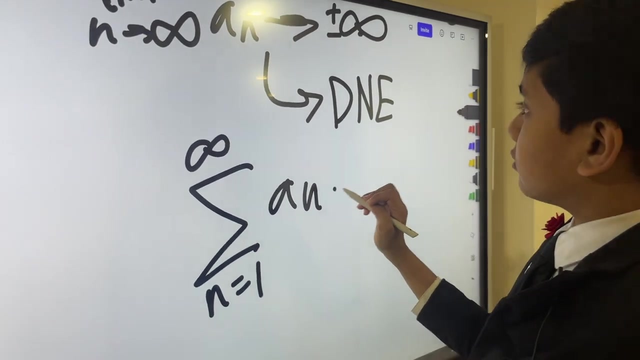 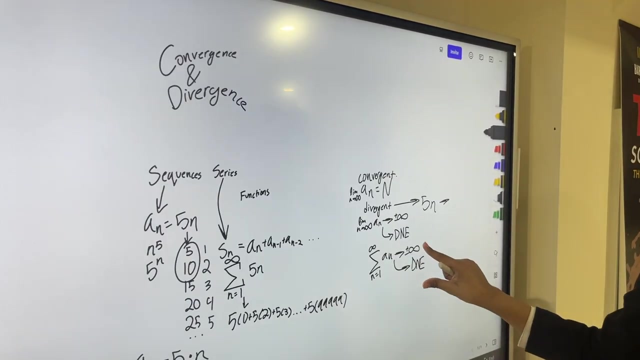 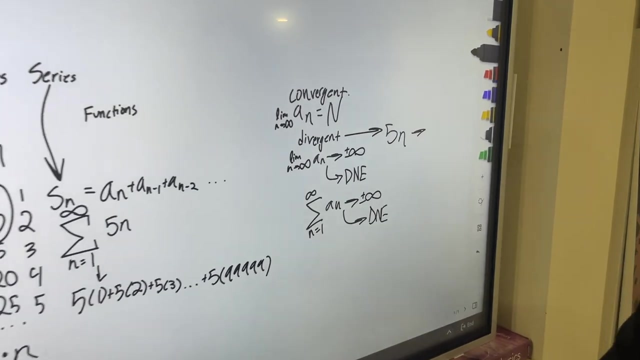 that Sn, or the sequence, the, This is equal to plus minus infinity, or dne or whatever. Because it's this. what this is basically saying is that the sum of all the terms will eventually approach infinity. Why? Because the sum of the terms just keeps getting bigger. 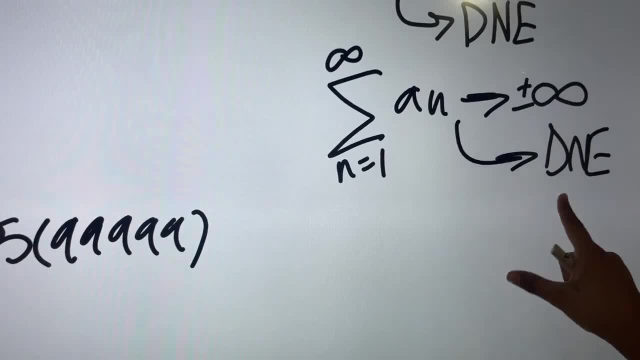 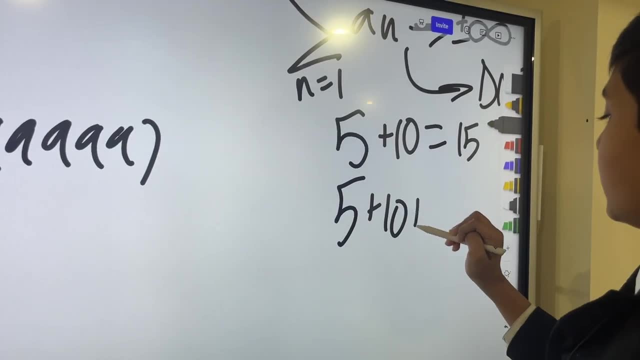 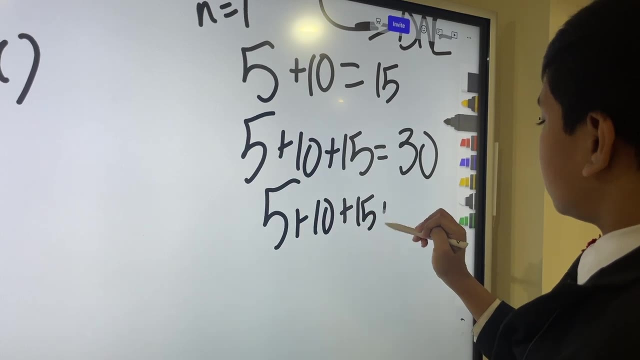 and gets bigger, And at an increasing rate too Like think about it: 5 plus 10, sum of the first two terms, 15, right. 5 plus 10 plus 15,, that becomes 30.. 5 plus 10 plus 15 plus 20,, that becomes 50. 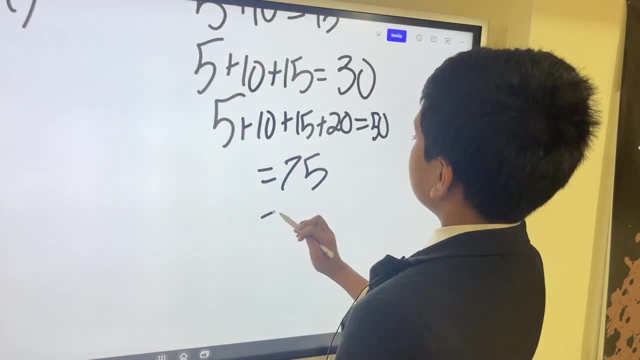 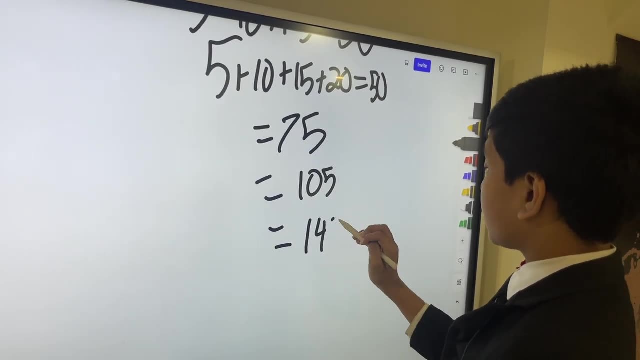 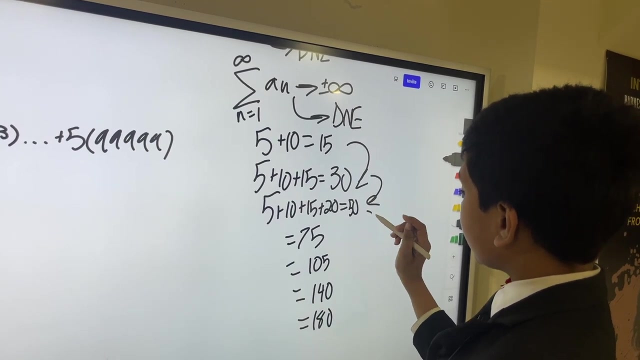 And even making it so odd, that's 75,, 105,, 105,, 140,, 180, and you can see it keeps growing and the amount it grows is actually bigger each time. That's because each term you add is bigger. 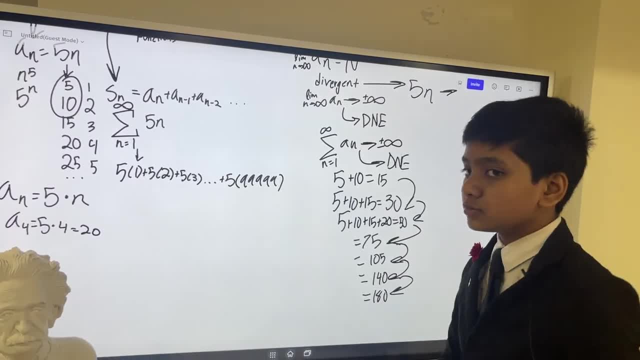 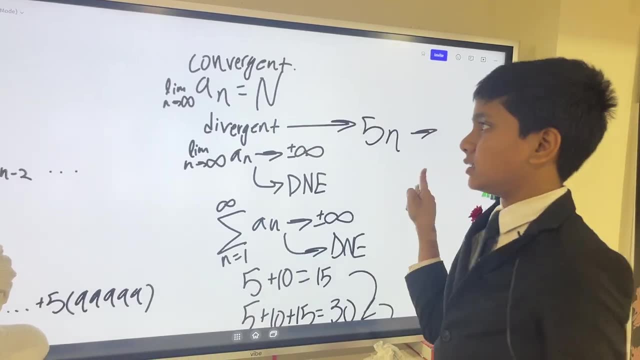 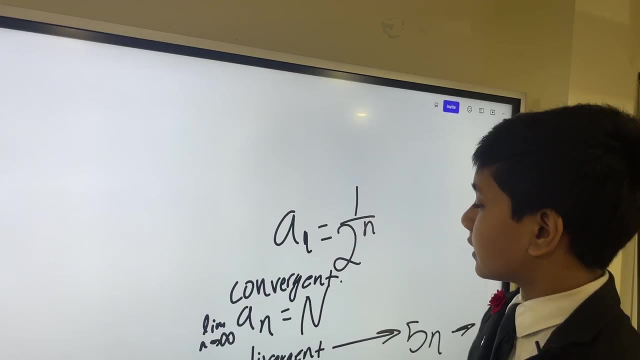 So that means that obviously the sum of the terms will approach infinity, Or in other words, it's divergent. Now let me show you an example of something convergent. So that would be something like this: It looks a little advanced, but trust me, it's not actually that hard. 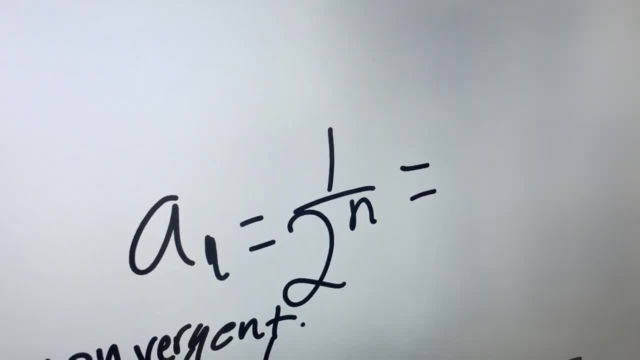 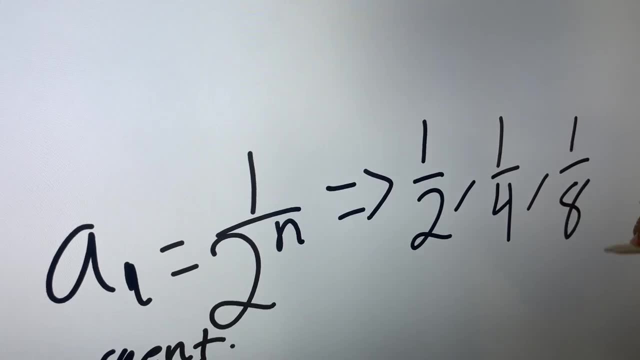 So 1 over 2 to the n, So that would be like 1 over 2, then 1 over 4, because 2 squared 1 over 8.. And technically, if you want it to be really technical, 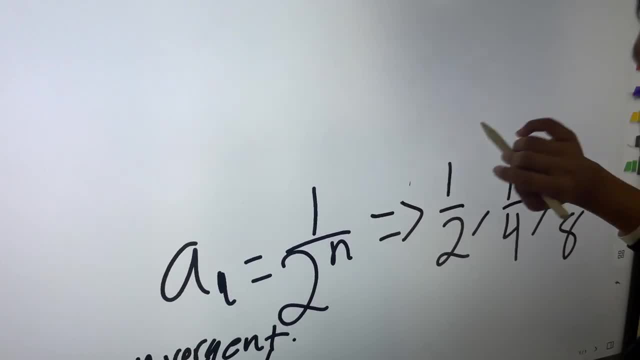 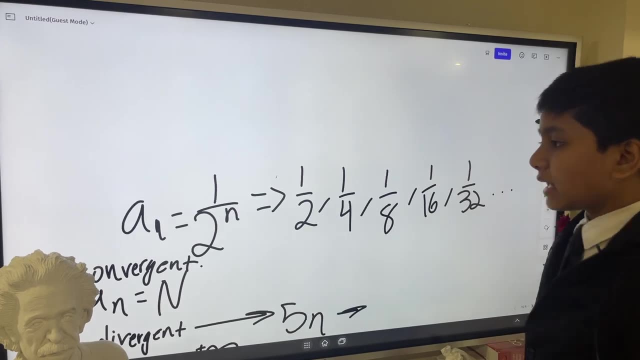 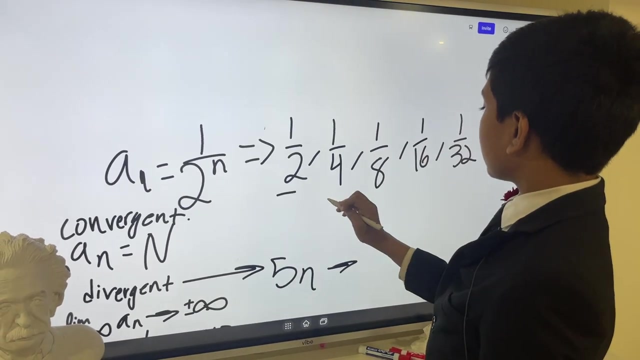 I guess you could include terms. no, let's not include 1 here, 1 over 8,, 1 over 16,, 1 over 32, etc. Now you might be asking: how is this convergent? Well, the thing is, the terms decrease every time. 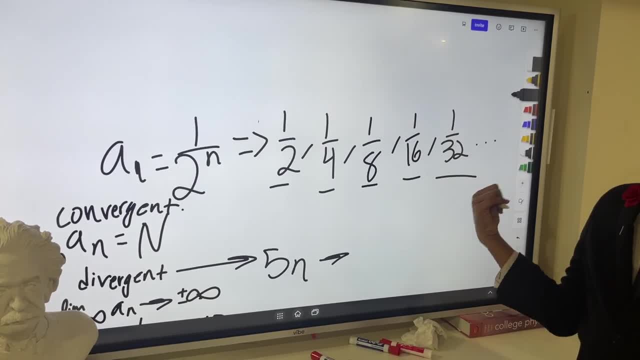 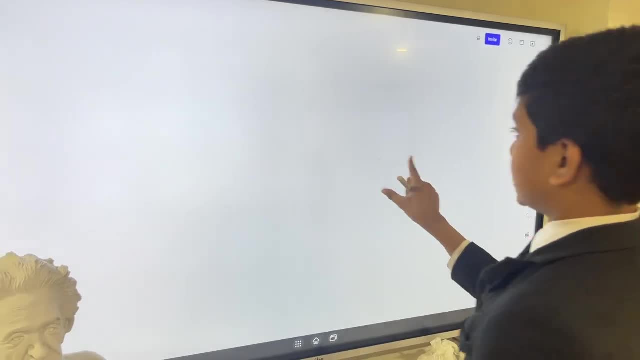 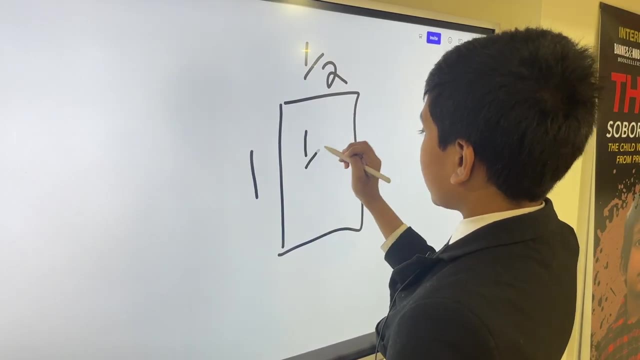 And I can't show you exactly how this is convergent. We'll do that in a future video. But basically I can show you this sort of geometric representation. Let's take a rectangle with size 1 half and 1. This has area 1 half right. 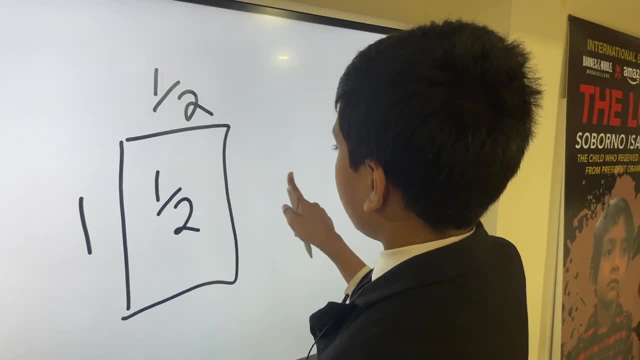 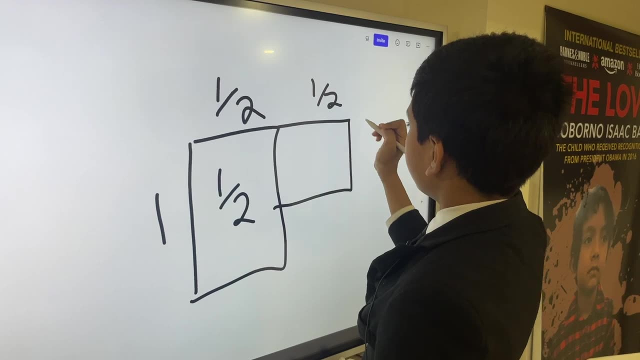 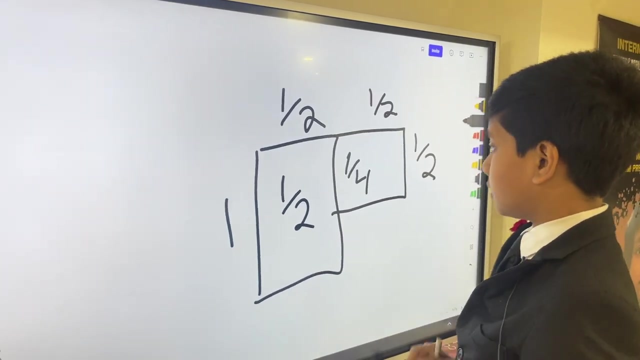 Then we have- Let's just take that- And we have now a rectangle with size 1 half and 1 half, making it 1 fourth. Now let's take that and make it 1 eighth. This is 1 fourth. 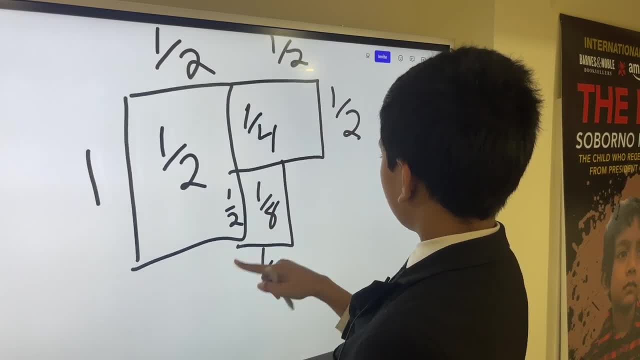 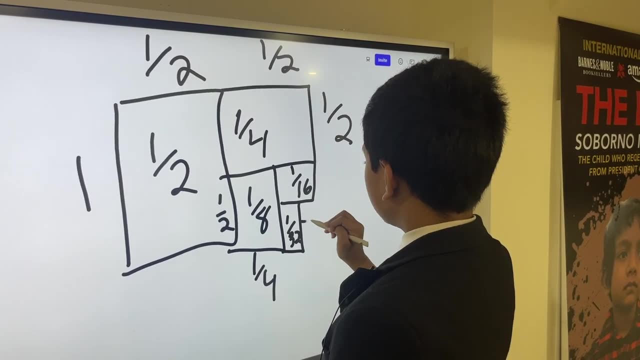 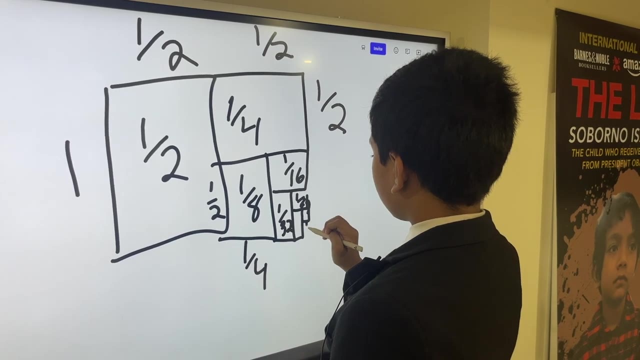 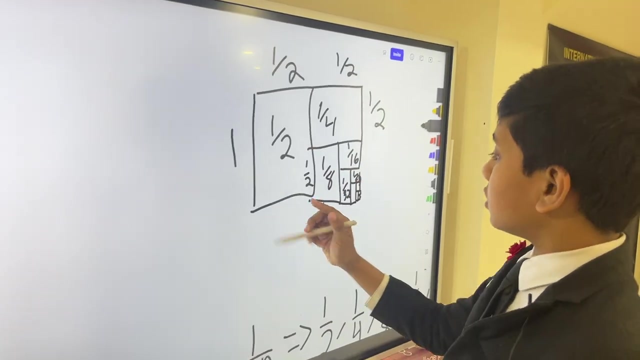 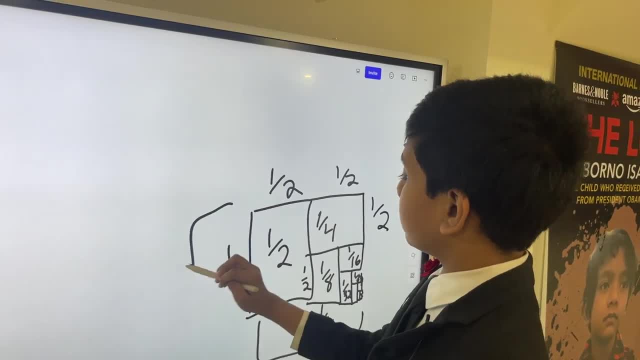 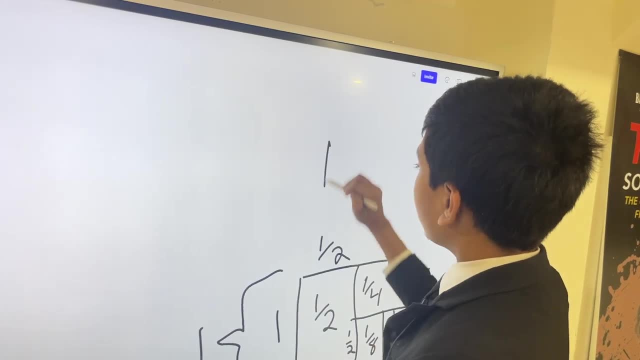 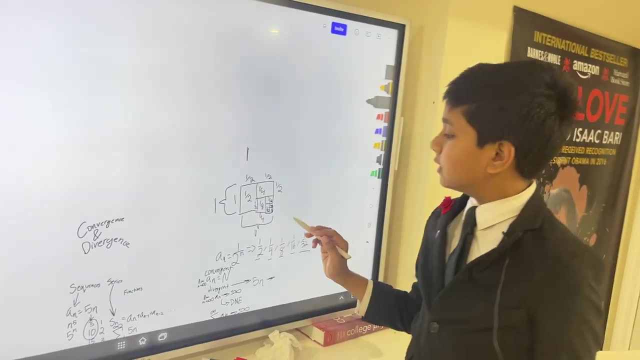 This side is going to approach 1.. And this side, as we know, is already 1.. So the area of this is just going to approach 1.- 1. When you add up all these terms, because they're decreasing in value, it will always end up in being 1.. 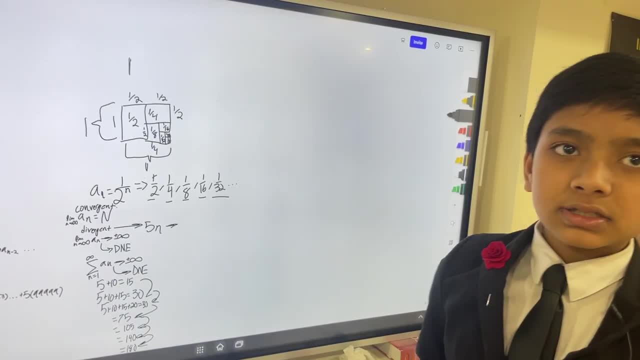 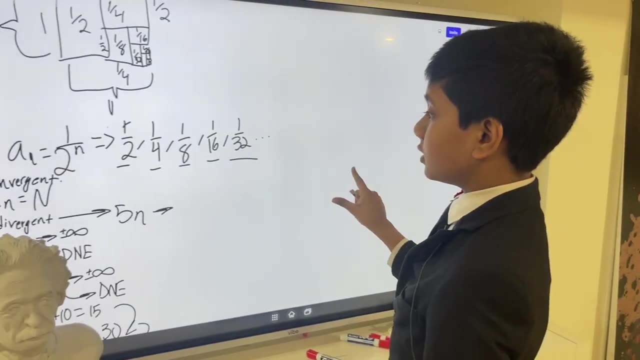 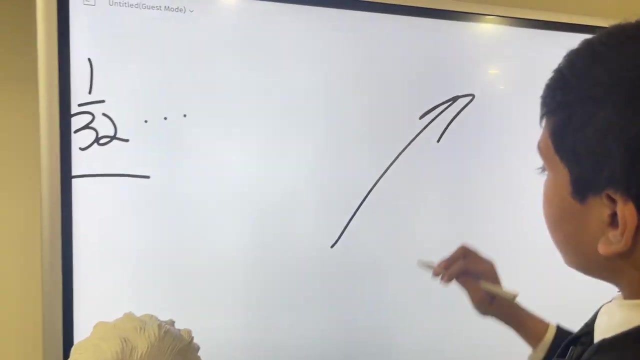 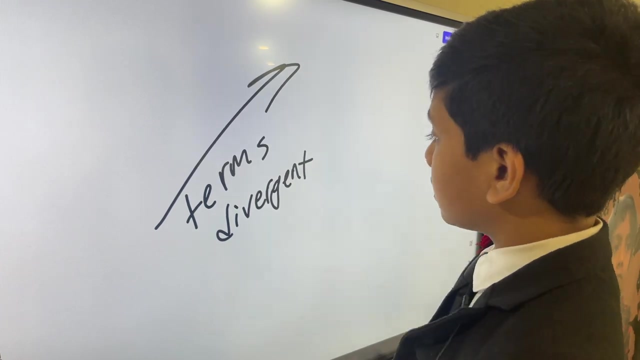 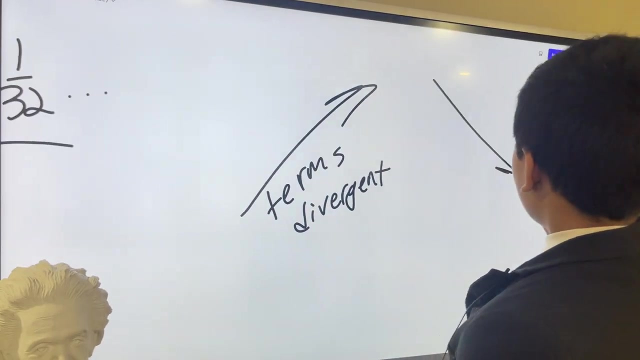 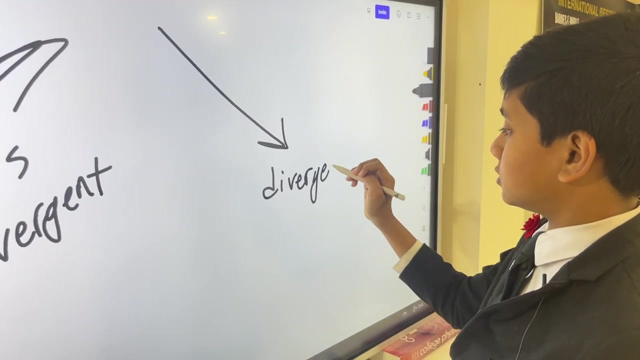 Okay, so just one quick way to test if it's going to become divergent. So basically, if the terms are increasing, then it's divergent. If the terms are decreasing, you might have either a divergent or a convergent one on your hands. 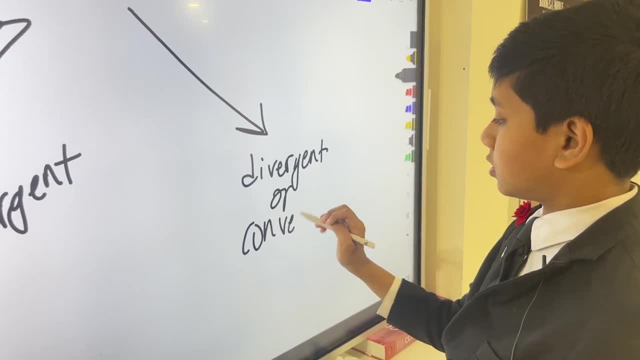 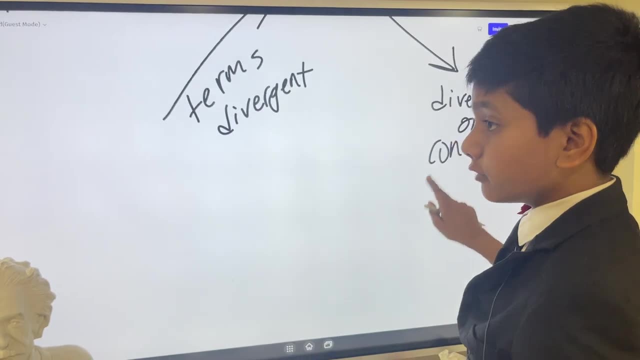 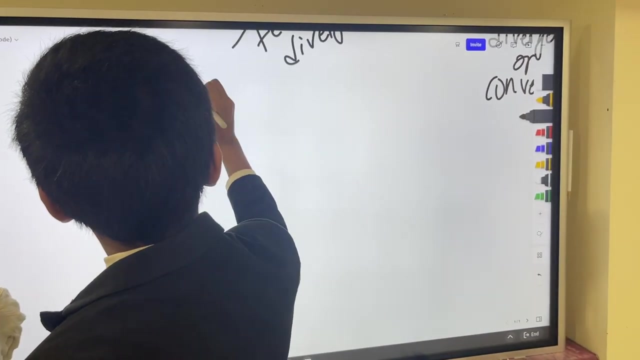 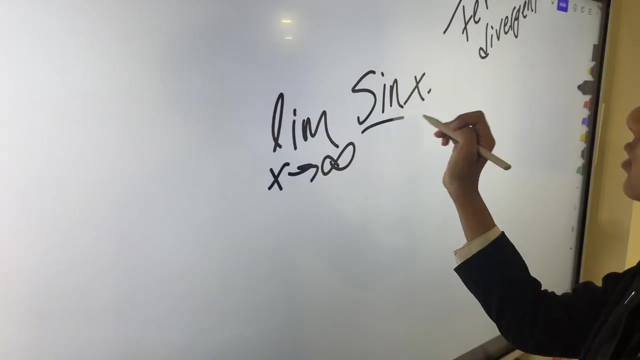 And now I'm going to show you one example that relates to all of this, And we're going to use a similar, related calculus rule while talking about this. So let's try to find the limit, as x approaches infinity, of sine x over x. 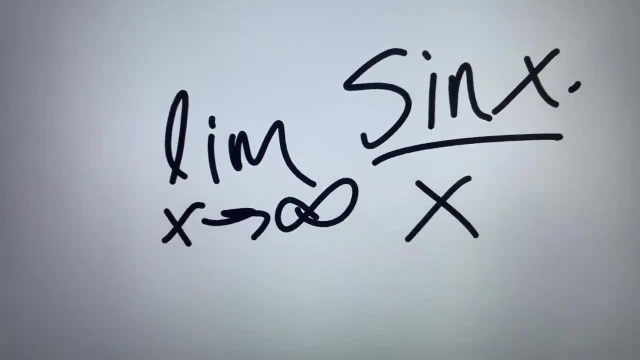 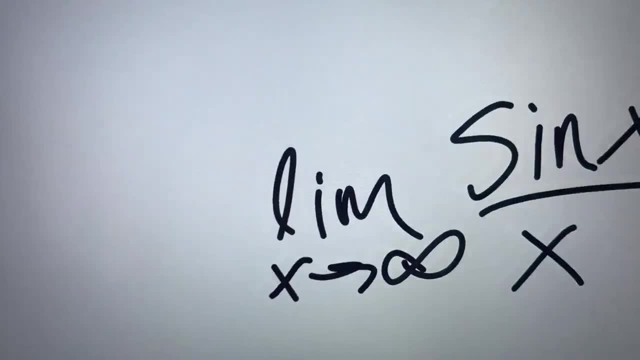 And this is much the same concept We're trying to find. We're trying to find the limit, as n approaches infinity, of something like this, which we could call a sequence. We could even say maybe this is a n equals sine n over n. 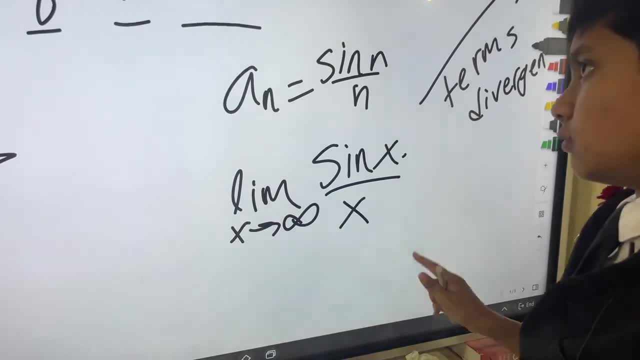 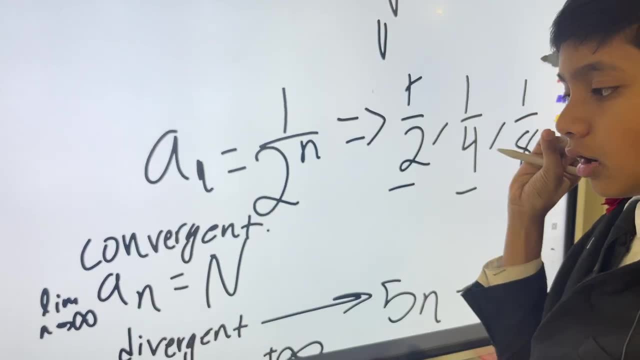 But how would we do this? Well, the conventional way of doing that. Oh wait, I just realized I can show you how this would end up being divergent. One way to test if it's going to be divergent is: 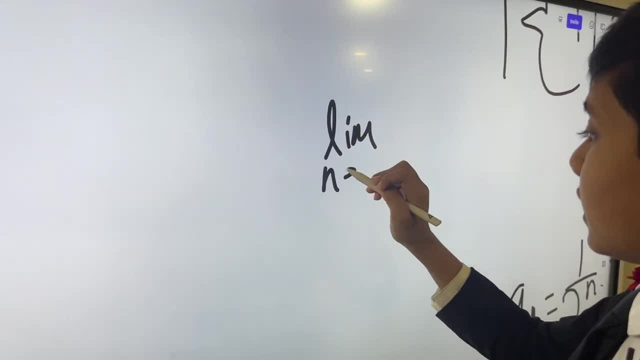 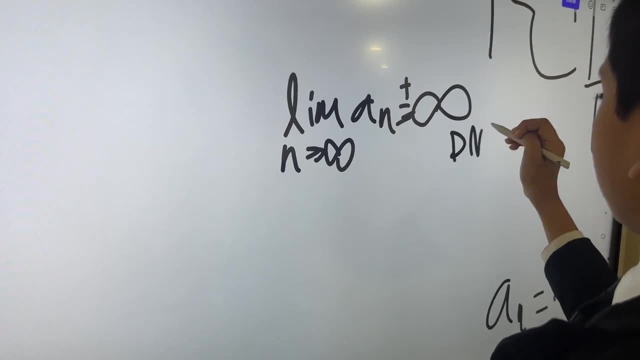 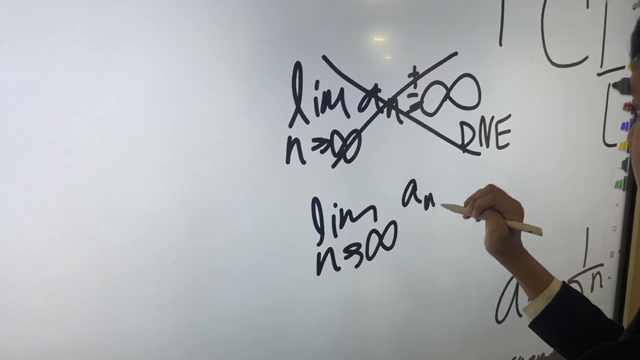 If the limit as n approaches zero. Well, if a of n is equal to infinity plus minus infinity, dn, e, whatever divergent, If it's equal to zero, you have either a divergent or convergent on your hands. 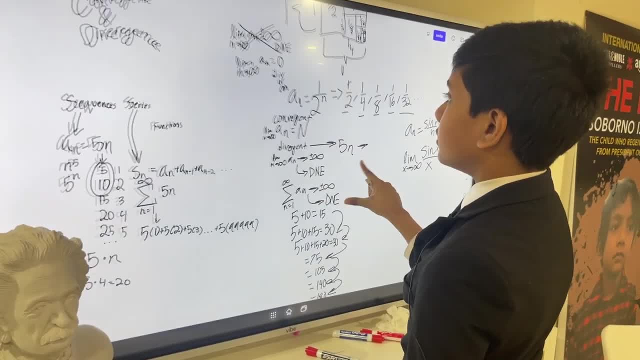 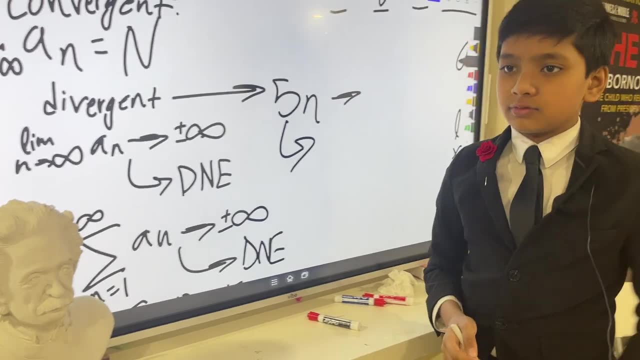 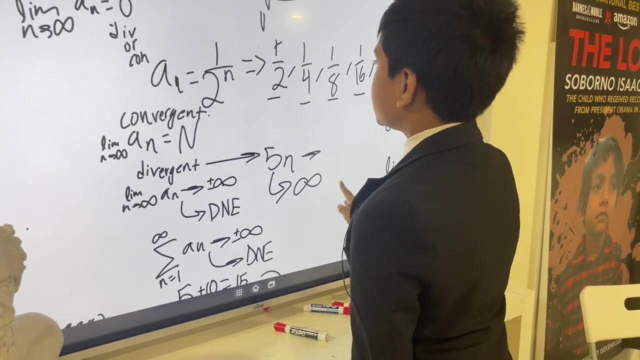 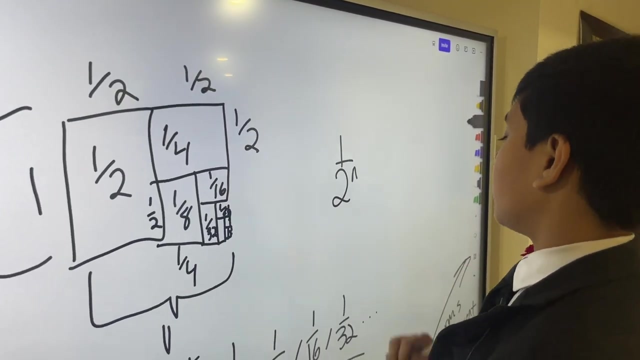 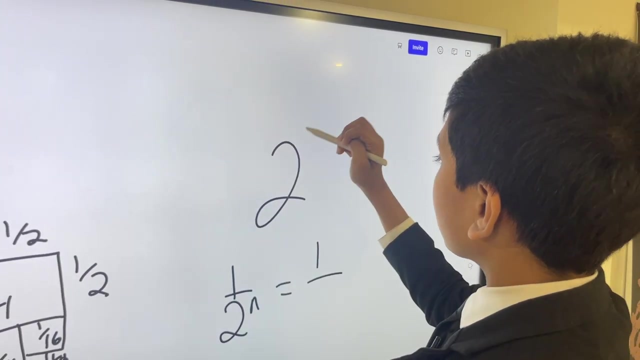 Now, as an example, we can just take the limit as this approaches infinity. but five times infinity, which we're basically We're substituting here for a very big, large number, is also going to be infinity. So something like 1 over 2n. the limit as that approaches infinity is going to become 1 over 2, raised to a large power. 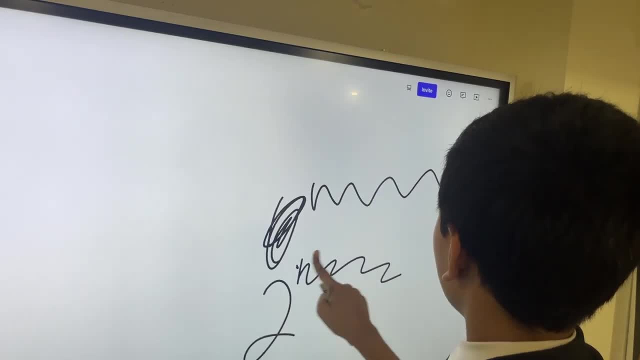 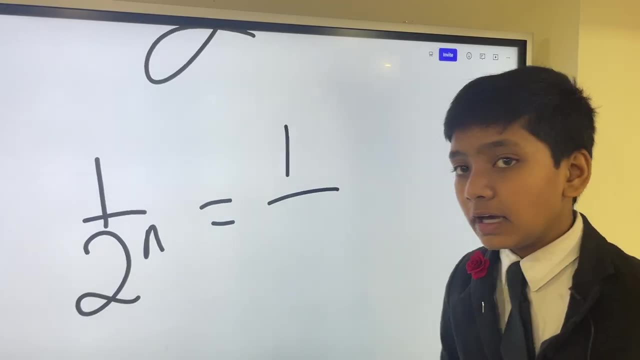 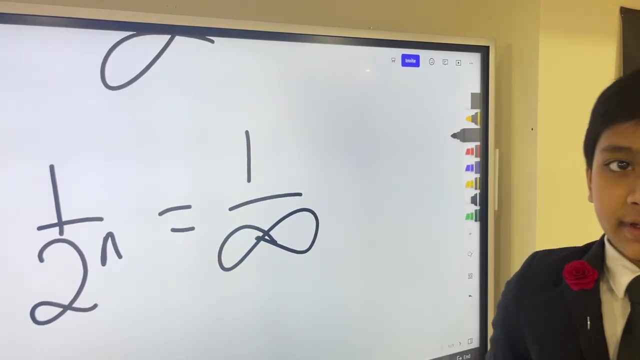 or really anything raised to a really large power is going to come out not just as large, but even larger. Think about that 2 to the 10 is already 1024.. So 2 to the infinity- we can just call that effectively infinity. 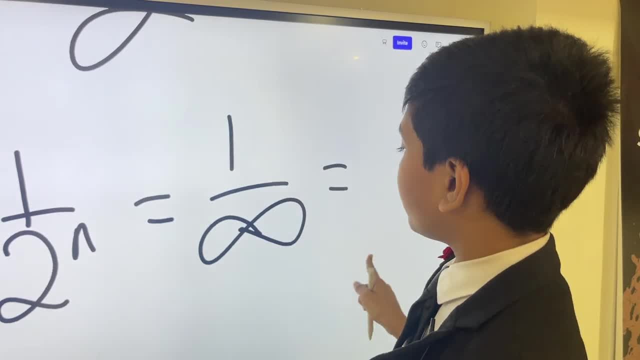 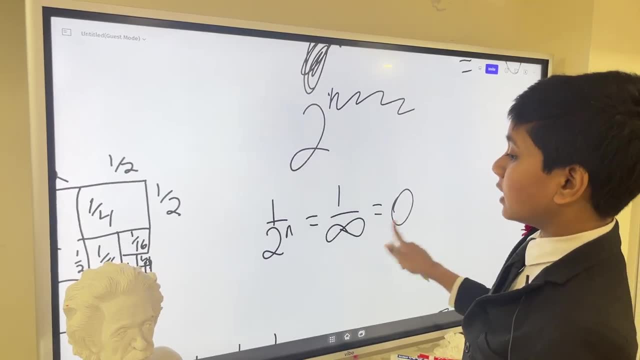 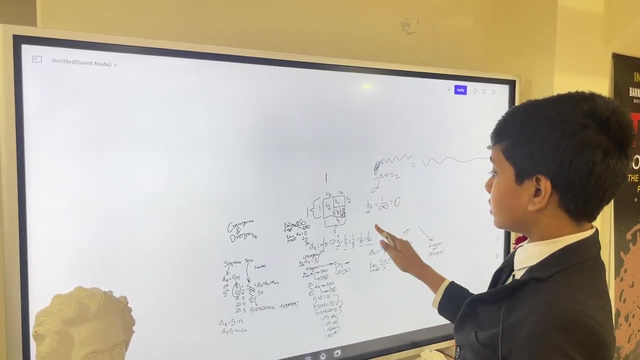 Substitution for a very big number. remember 1 over infinity is effectively zero. Remember very big number And if you think about it, it makes sense. The numbers keep getting smaller. they effectively get closer and closer to zero. So since 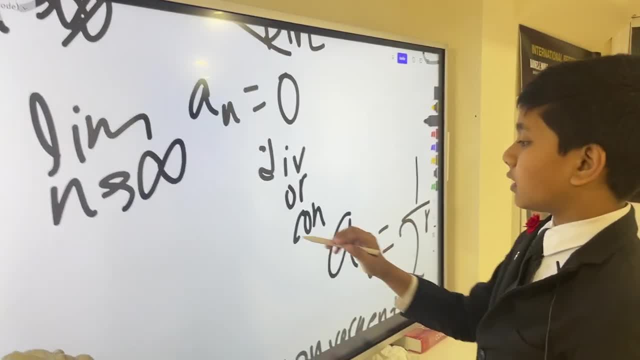 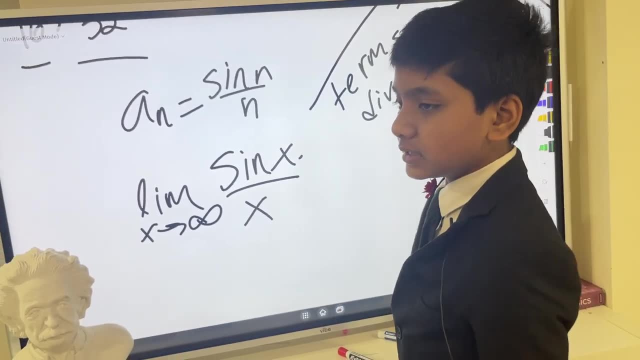 This approaches. This approaches zero. it's either a divergent or convergent, and we've discovered that it's a convergent. We can use this divergent-convergent strategy in order to find out if this is divergent or convergent. 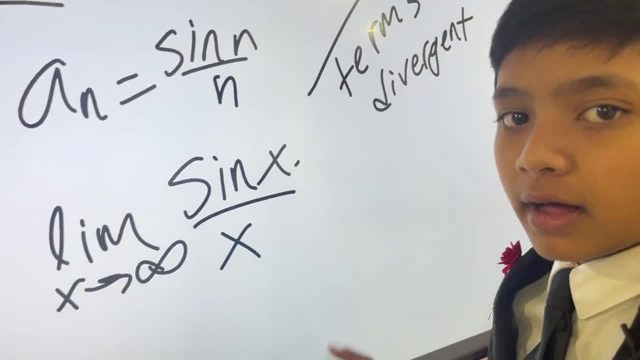 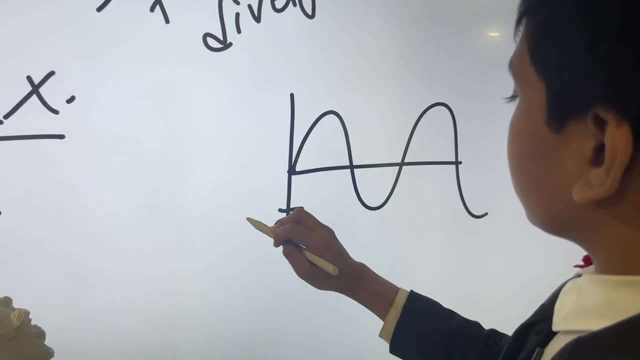 So sine of x over x? how can we do this? Well, let's think about the function. sine of x Oscillates between minus 1 and 1, right, But we know it's always between these lines which we can essentially. 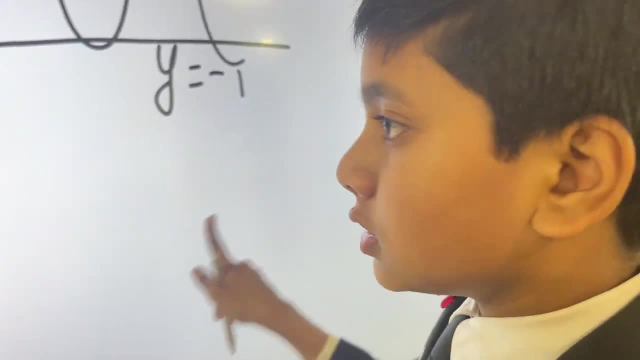 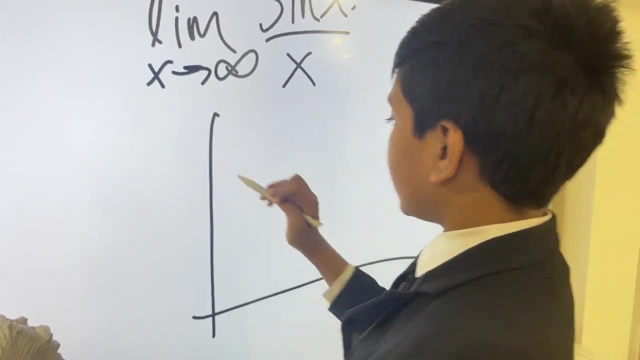 We can say: oh, y equals 1 and y equals minus 1.. So now we know We can talk about the squeeze theorem for a little bit. So let's say we have a function f of x on the top over here. 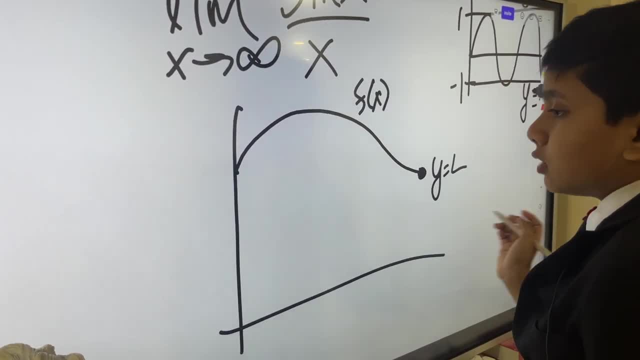 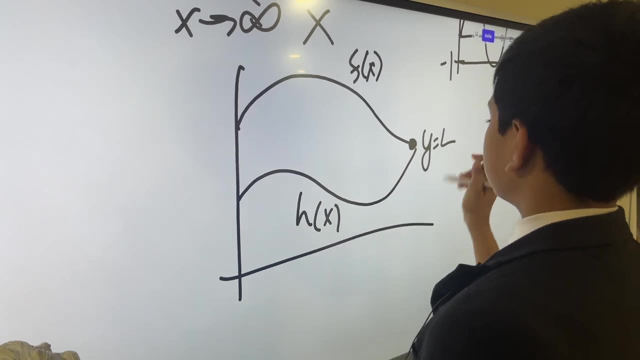 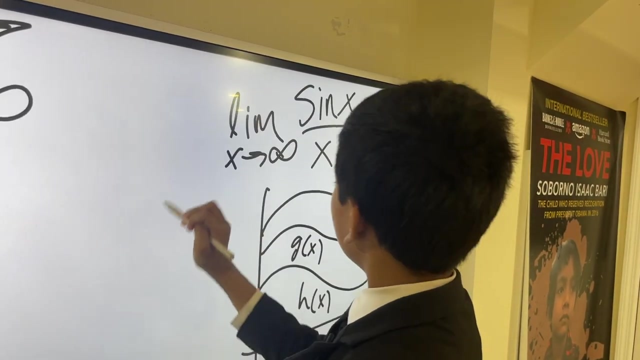 approaching, let's say, y equals l, And we have this function now here: h of x, which is also approaching y equals l. Then if g of x over here is stuck in the middle, so given this definition, Sorry, let's rewrite that. 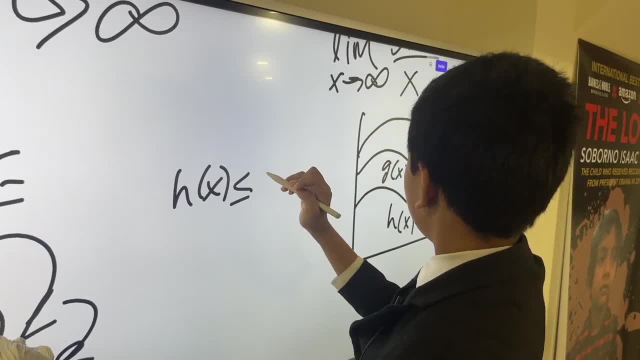 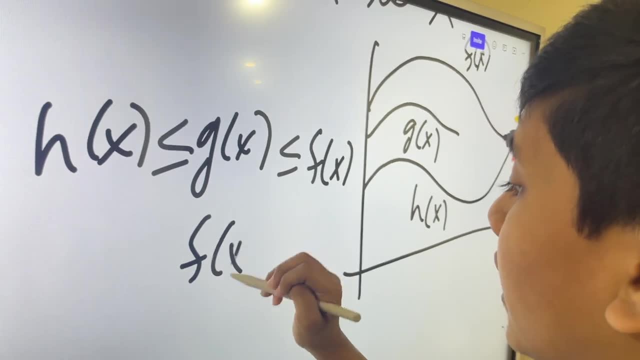 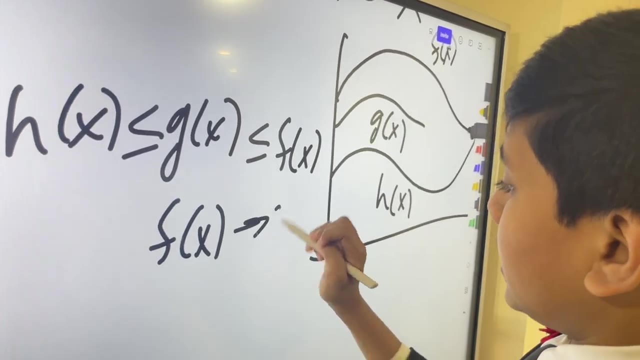 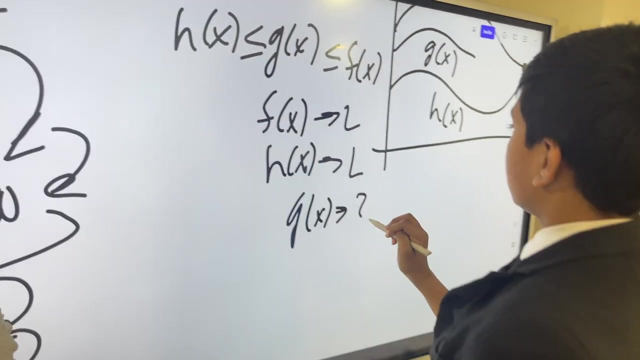 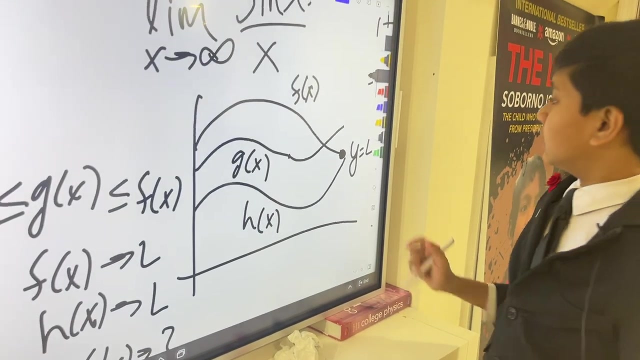 So, given this definition And the fact that f of x is approaching l And h of x is also approaching l, What will g of x approach? Well, the obvious answer is: it can't go anywhere above l, because that would be violating the less than f of x rule.